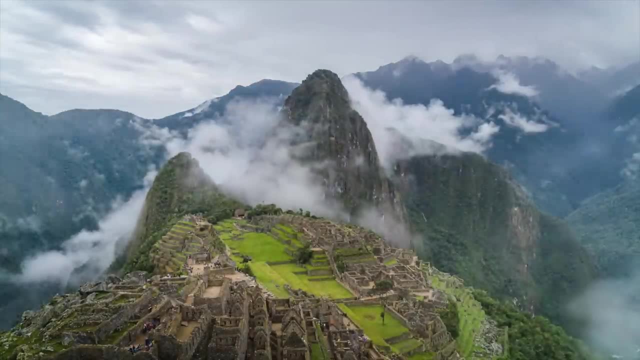 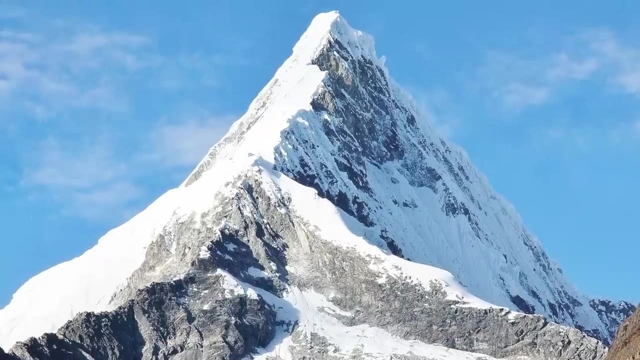 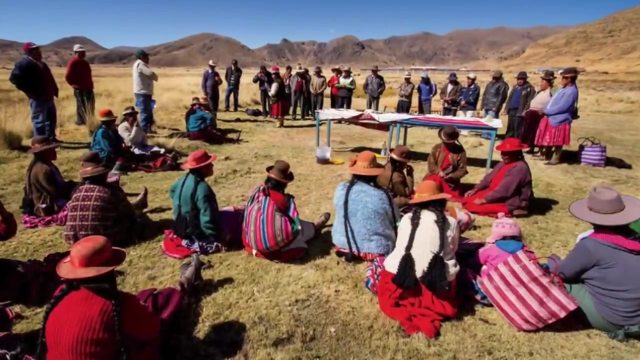 you are probably already aware, is where the famous Inca town, Machu Picchu, is located. You've probably seen another famous Peruvian mountain without realizing it. This mountain was the inspiration for the newer Paramount Pictures logo: The natives of the Andes Mountains, specifically. 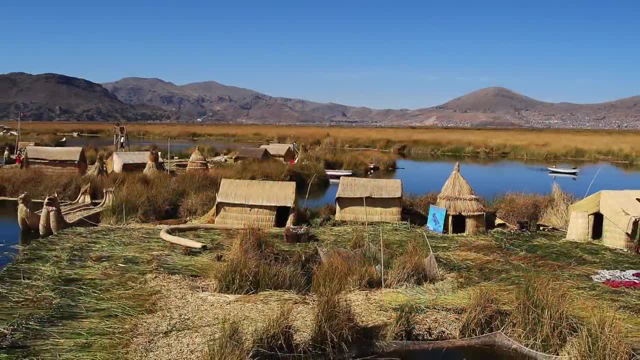 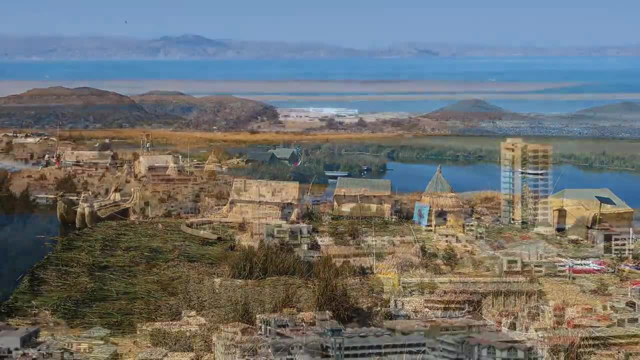 those of a region shared with Bolivia called the Altiplano, also known as the Andean Plateau, have adapted to the thin air by developing an ability to carry more oxygen in each red blood cell, which allows them to breathe at the same rate as normal people who live at sea level. But the Andeans 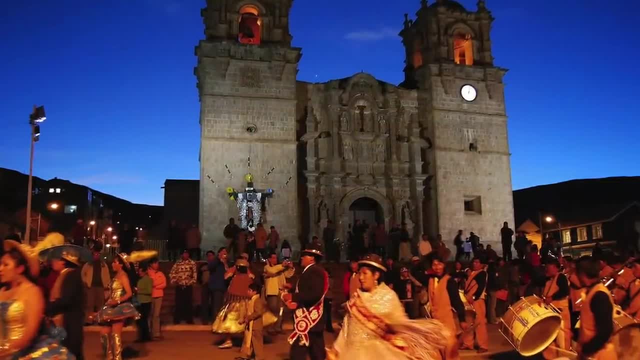 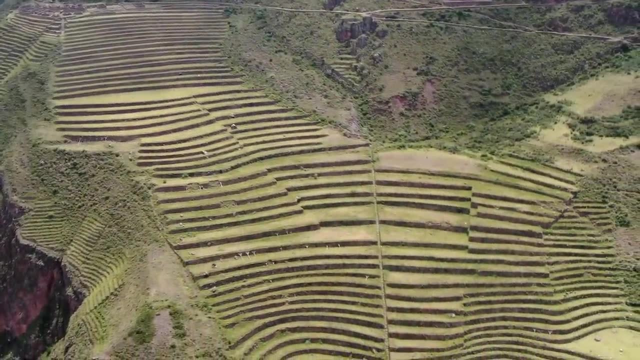 have the ability to deliver oxygen throughout their bodies more effectively than people at sea level do. On top of just being natural superhumans, the Peruvians adapted to the mountainous landscape with terrace farming, And they grow different crops at different levels of elevation. 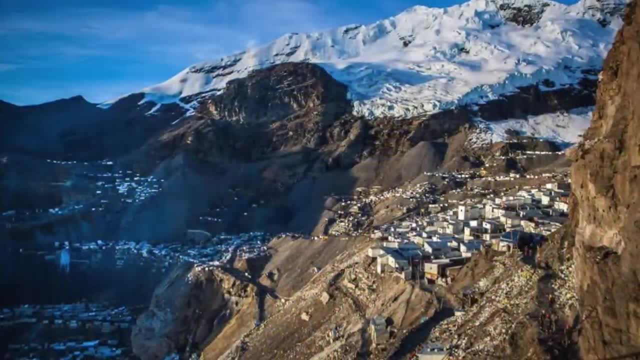 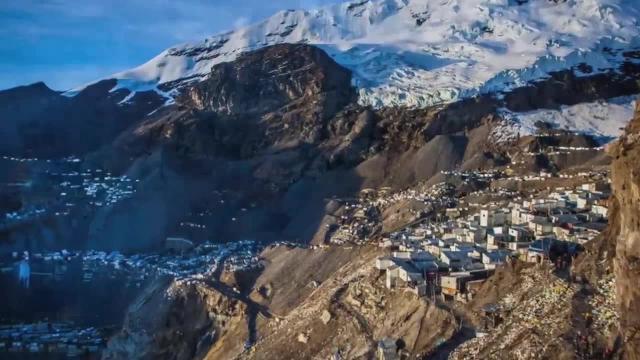 depending on what grows best. These mountains are home to the highest town in the world. It sits at around 5,100 meters or 16,700 feet in elevation. The town sits next to a gold mine, so as the price of gold grew in the first decade of the 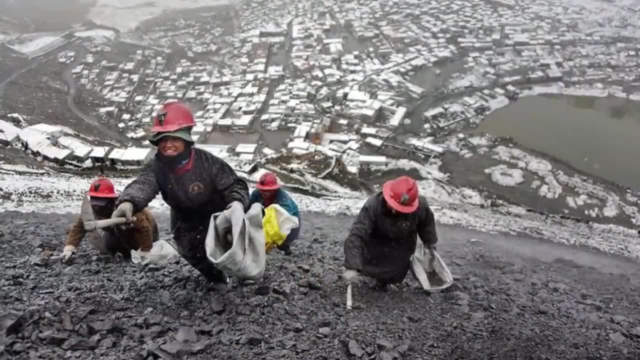 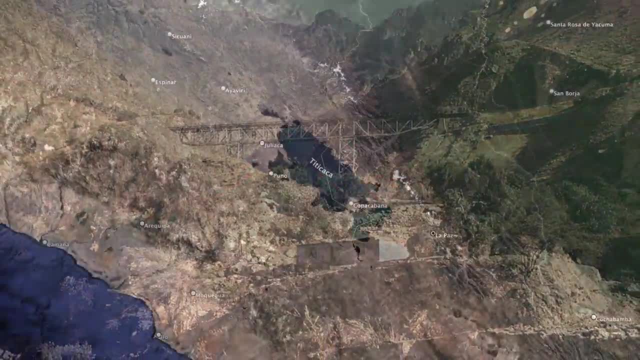 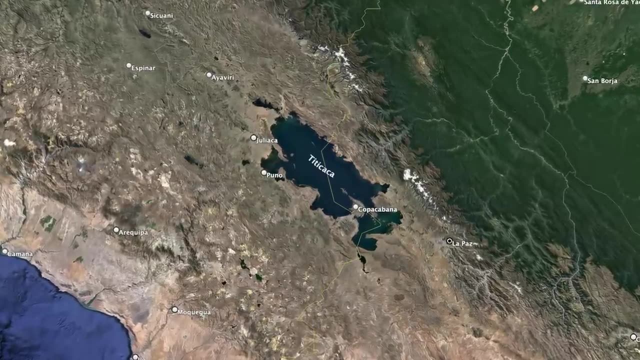 21st century, a few small camps quickly rose to around 30,000 people. Within the Peruvian Andes is also the second highest railroad in the world. As far as natural wonders go, Peru is home to the world's highest major body of navigable water. Its name is Lake Titicaca. 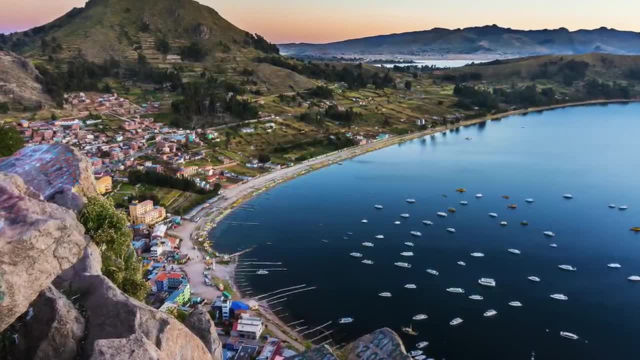 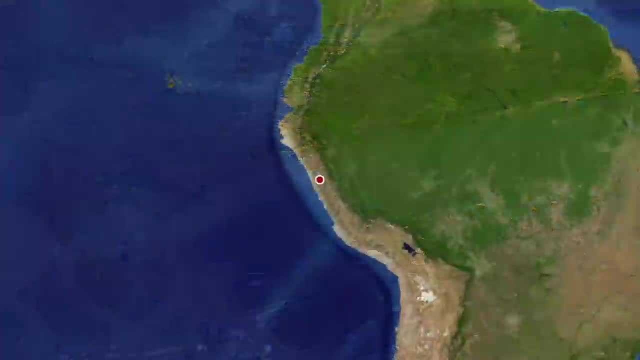 This lake is shared with Bolivia and sits at 3,800 meters, or 12,500 feet in elevation. It is also the largest lake in South America, But maybe the weirdest random fact about the Peruvian Andes is that it is home to the point with the weakest gravity on Earth. 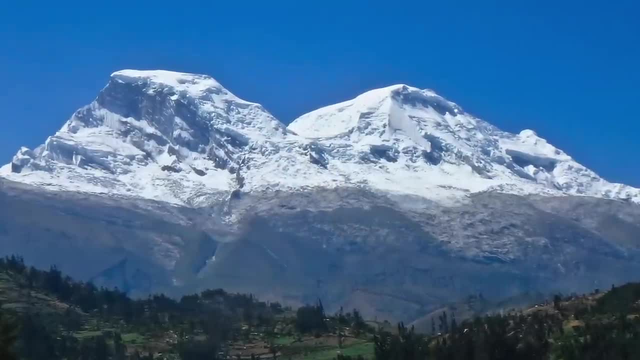 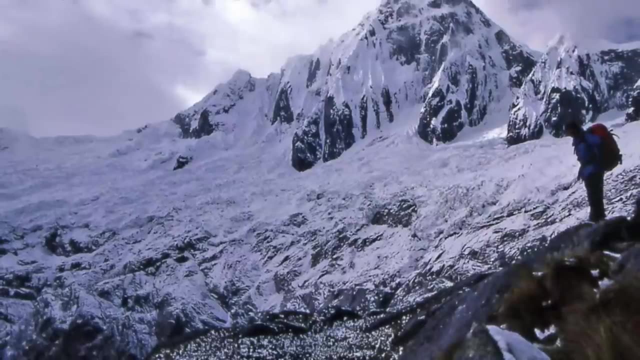 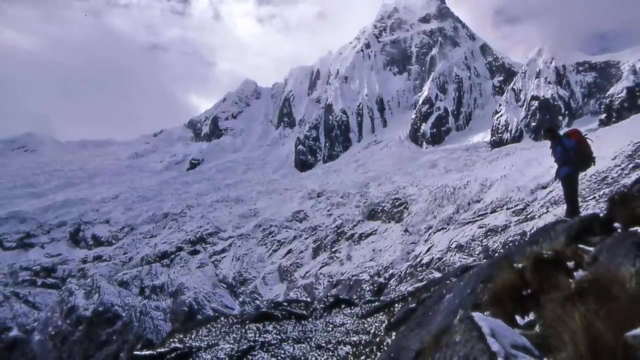 This would be the highest southern summit of Huascaran, the highest point in Peru, the northern Andes and in all of Earth's tropics. It stands at 6,768 meters or 22,205 feet. Its gravity is around 0.7 percent lower than the place with the strongest gravity. 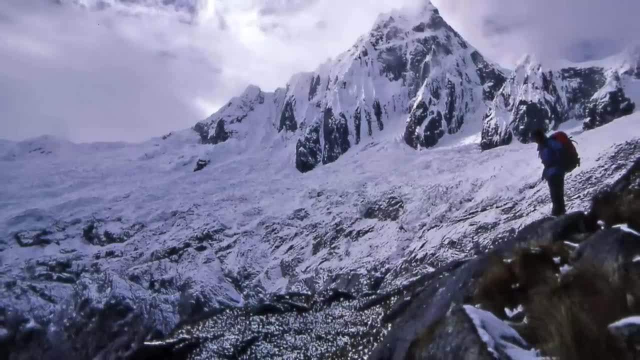 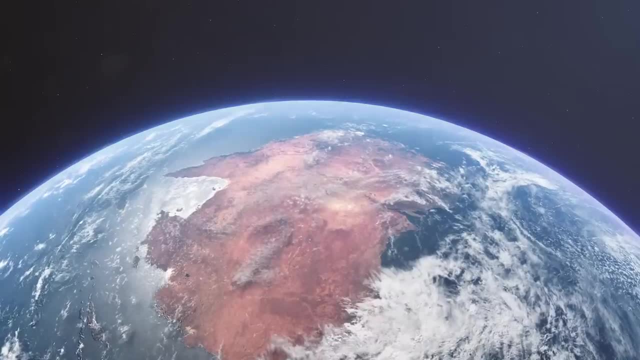 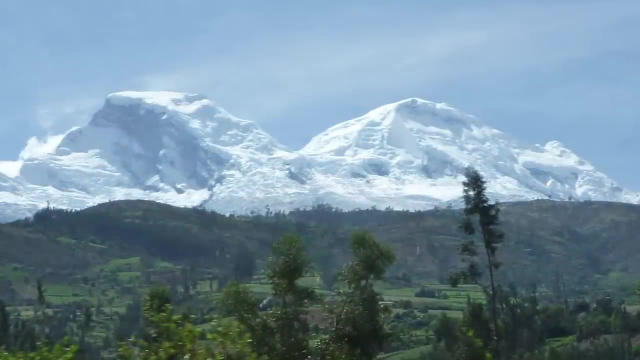 which is at the surface of the Arctic Ocean. The variation in gravity is due to a combination of factors. This includes Earth's rotation and its resulting equatorial bulge, which make gravity around the equator slightly weaker, altitude and varying densities of Earth's crust. Huascaran's. 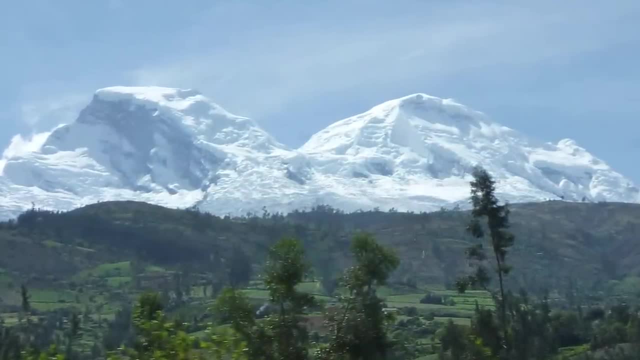 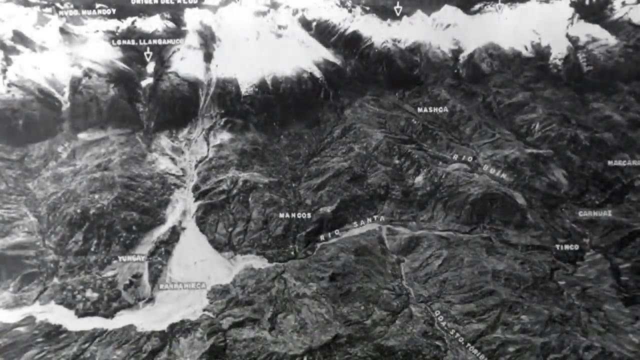 gravity is lower because it sits close to the equator and its summit is high in elevation. I've left a link in the description to a video that explains this in more detail. The mountain is also responsible for two of the three most important lands in the world, among which the 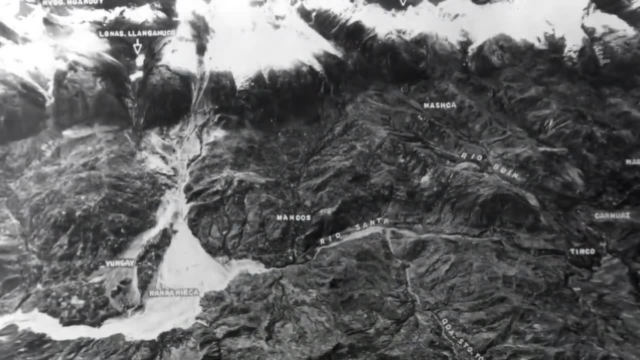 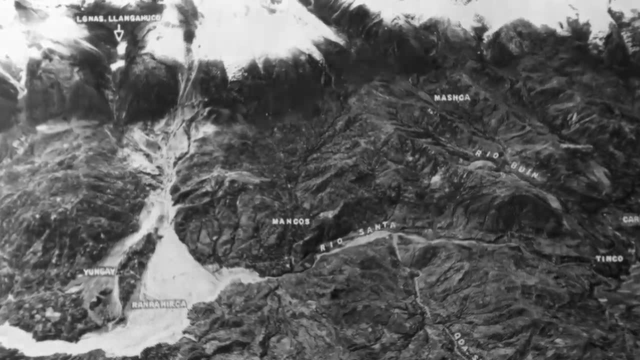 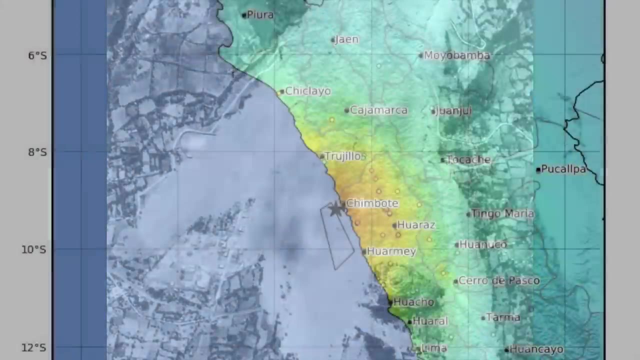 two of the three deadliest avalanches in recorded history, both of which happened less than 10 years apart: One in 1962 that killed approximately 4,000 people, and another in 1970 that killed over 20,000 people. This avalanche was the result of a 7.9 magnitude earthquake. The earthquake. 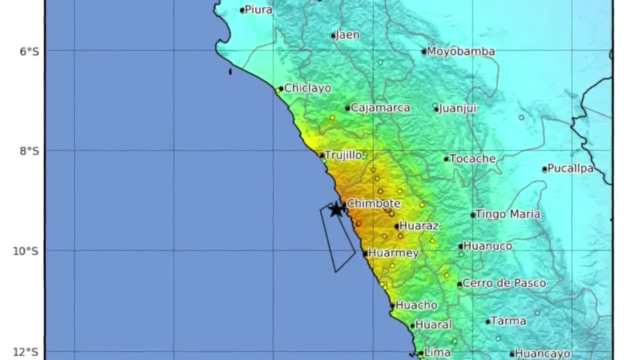 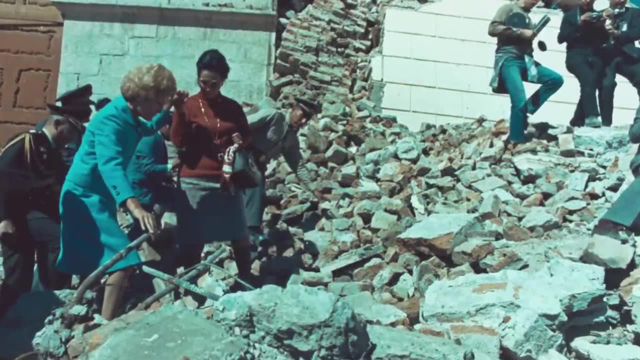 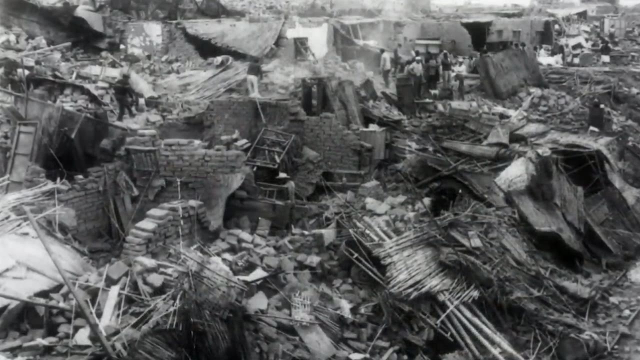 affected an area of about 83,000 square kilometers, an area larger than Belgium and the Netherlands combined. In total, the earthquake resulted in the deaths of around 70,000 people, caused 50,000 injuries, destroyed roughly 200,000 homes and buildings, and left approximately 800,000 people. 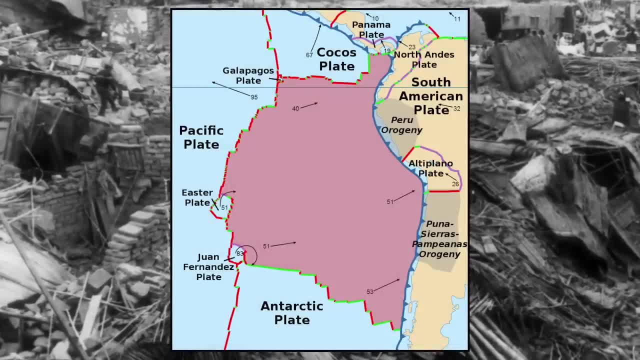 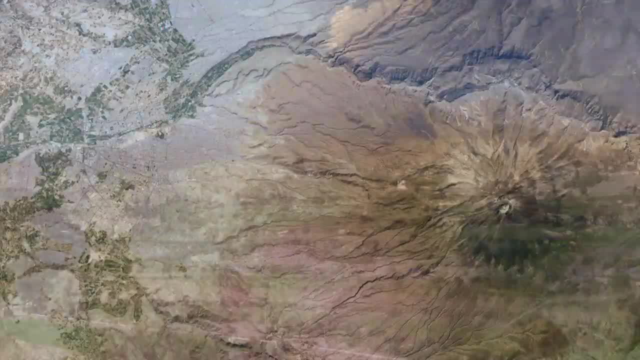 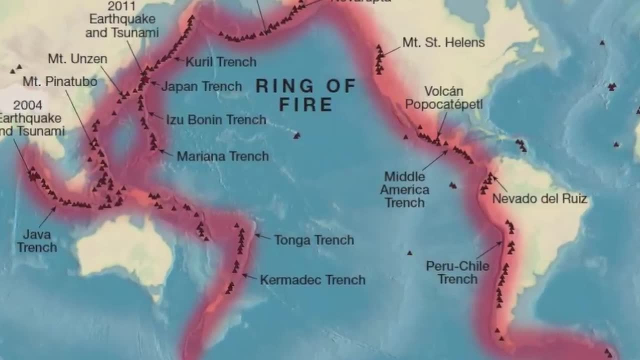 homeless. The country is prone to earthquakes because of the convergent boundary that the country sits on. This has also created volcanoes. Peru has 31 volcanoes, 16 of which are active. This zone is part of the larger region called the Ring of Fire, a horseshoe-shaped belt around 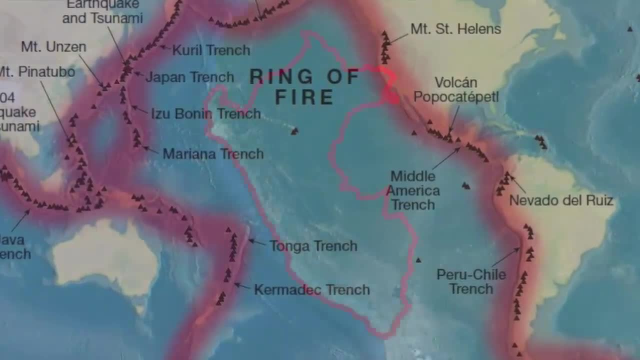 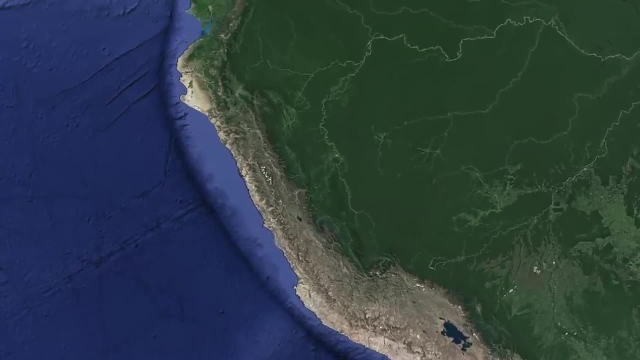 the Pacific Ocean, where volcanoes and earthquakes are common. The Andes create what is called a rain shadow effect: Moist air is blown from the east. That moisture essentially becomes trapped in the mountains, resulting in the arid landscape on the other side, Though. another reason for the 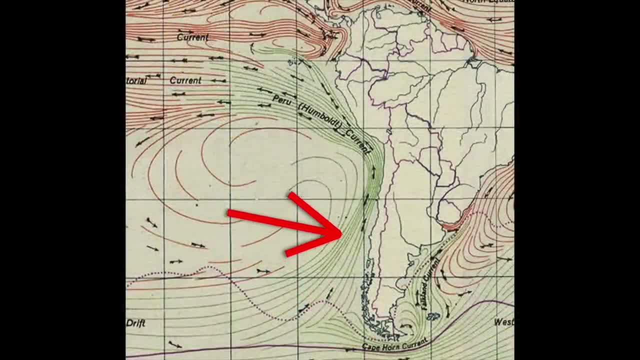 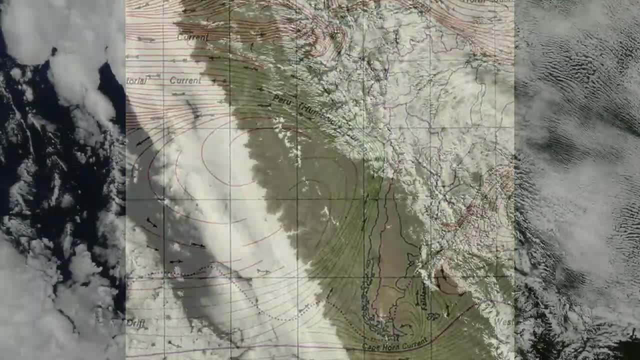 aridity is the Humboldt Current, also known as the Peru Current. Air moving north is cooled by the cold water current conditions that result in low precipitation, Though, interestingly, it generates fog. This also inhibits the flow of water, which is why it is called the Humboldt Current. 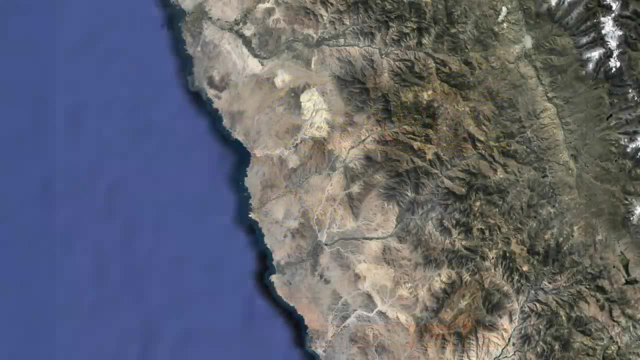 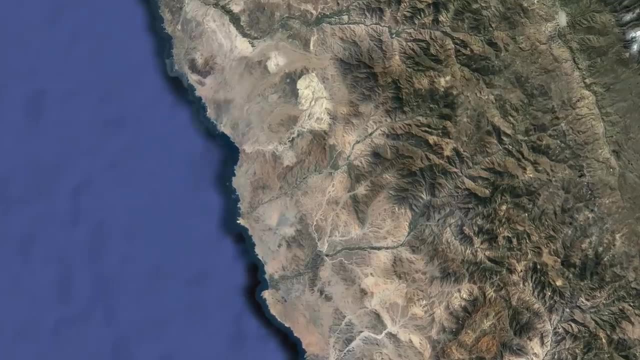 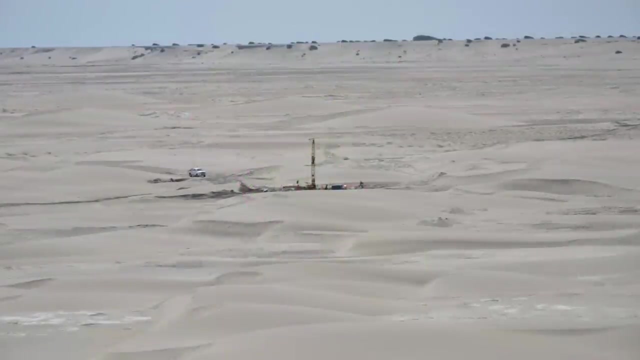 It makes little difference. but what parts of the arid coast belong to what desert are different depending on who you ask. Some say the entire Peruvian desert is the Sechera, while others say that it meets the Atacama within its borders, The lowest point in Peru, and all of the southern tropics, for that matter, is located within the desert. The lowest point is 34 meters or 112 feet below sea level. The Peruvian desert is also home to the famous Nazca Lines, Because of its isolation and the dry, windless, stable climate of the 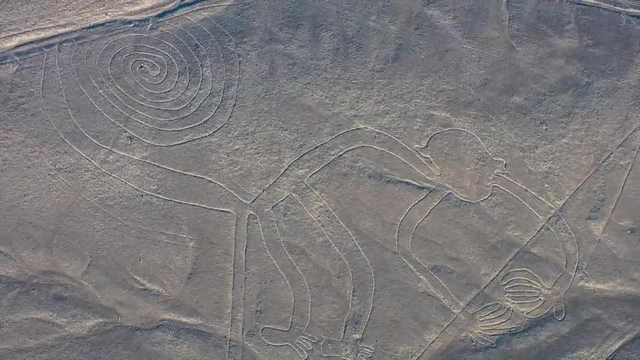 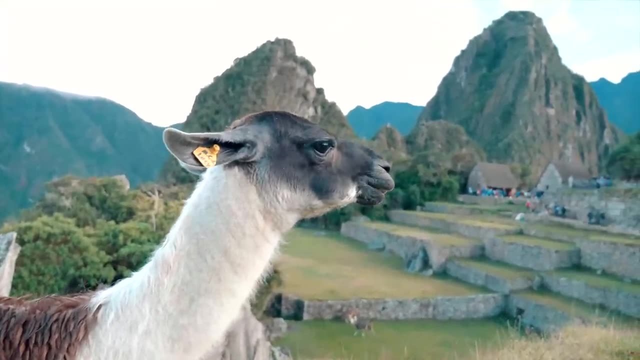 plateau, within the desert, where the lines are located, they have mostly been preserved naturally. This climatic diversity of Peru has, of course, resulted in diversity of plant and animal life. Peru is the fifth most biodiverse country in the world. The only countries with more native plant. 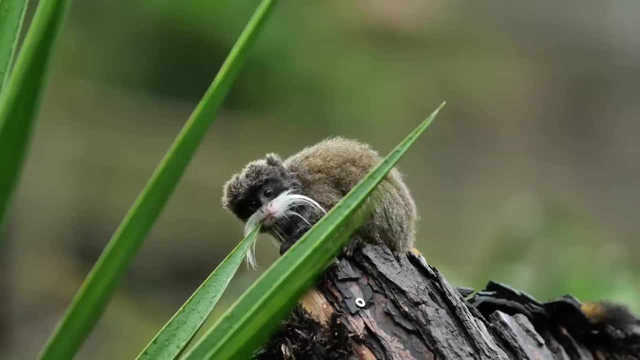 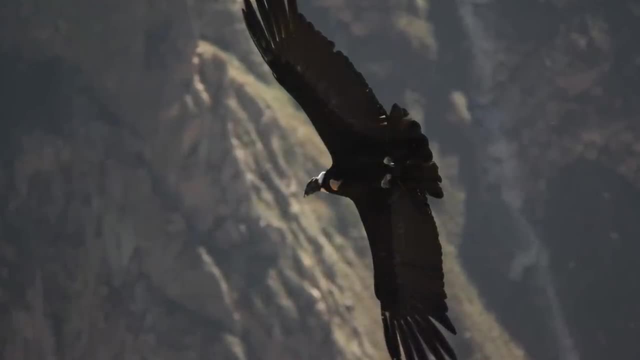 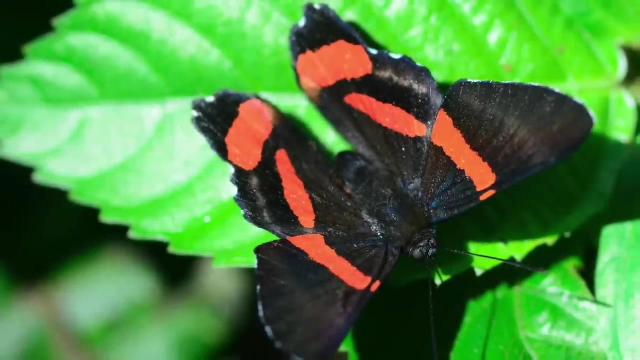 and animal species are Brazil, Indonesia, Colombia and China, two of which are significantly larger countries. Peru is home to 18.1% of all bird species on Earth. The only country with more is Colombia at 18.3%. There are more than 17,000 species of butterflies in the world, And Peru holds the largest number. 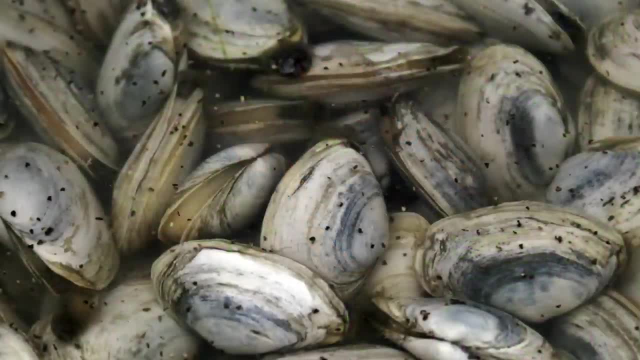 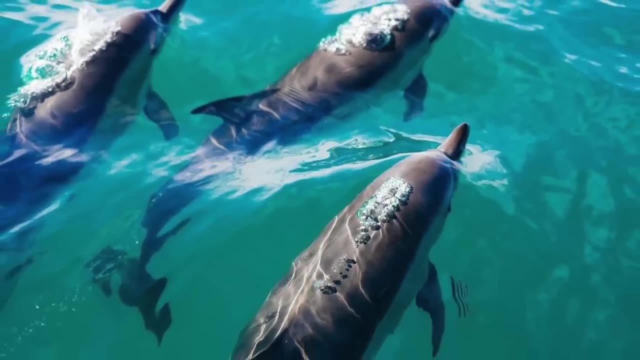 of them. with more than 4,000 species, With over 700 different varieties of fish and 400 varieties of shellfish, the waters off Peru's coast is a highly diverse ecosystem. on its own, It's also one of the most successful. 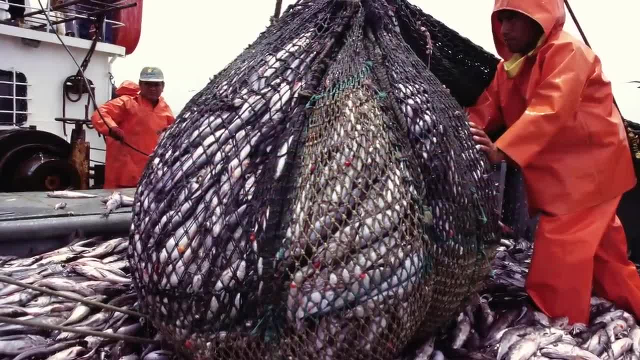 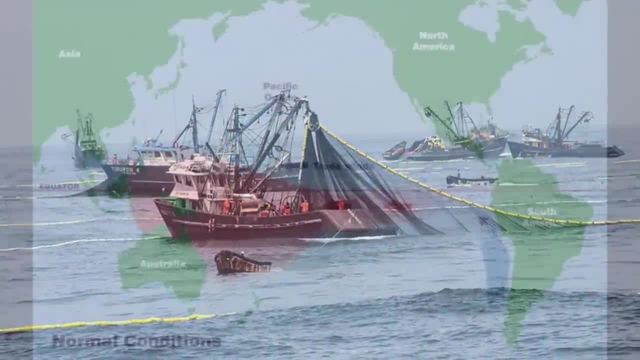 commercial fisheries in the world. This is largely due to the previously mentioned Humboldt Current. The current causes a welling up of marine and plant life on which the fish feed, But every three to seven years the weather event El Niño negatively impacts fish abundance and distribution. 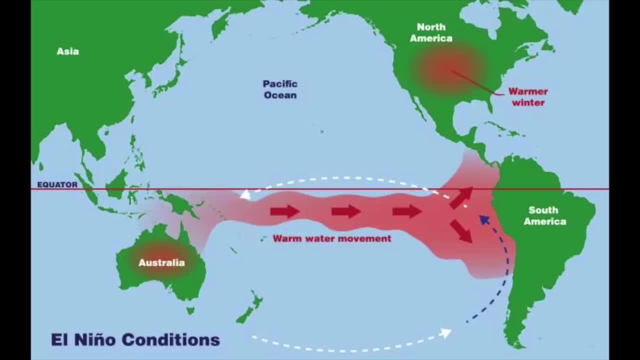 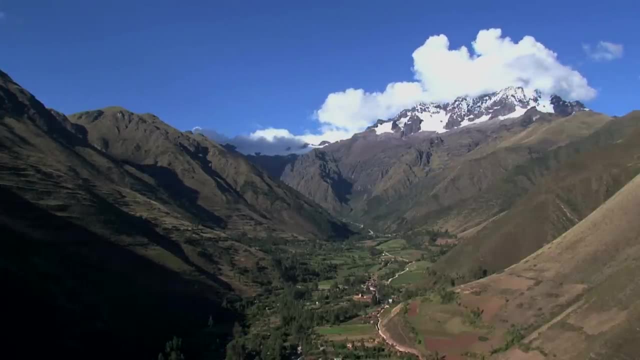 El Niño is a band of warm ocean water that disrupts the flow of the Humboldt Current, destroying the feed for fish. Peru has a lot of other interesting features relating to its physical geography. Here are a few not already mentioned: A river that reaches a depth of 1,000 feet. A river that reaches a depth of 1,000 feet. 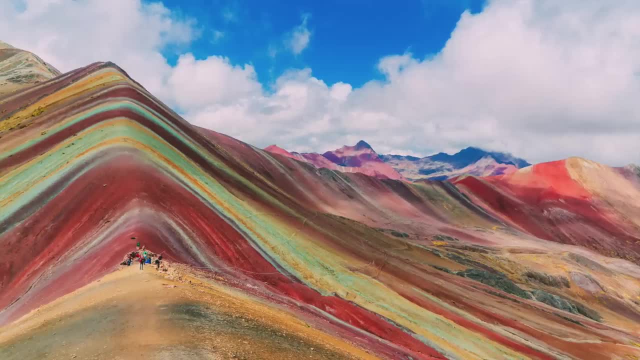 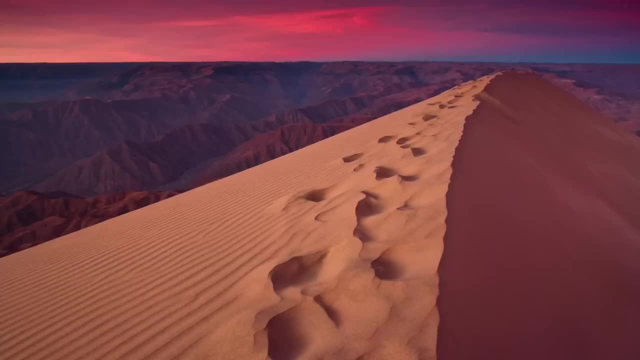 A canyon that is nearly twice the depth of the Grand Canyon. A canyon that is nearly twice the depth of the Grand Canyon, A canyon that is nearly twice the depth of the Grand Canyon, The second highest sand dune, The world's largest left-hand wave. 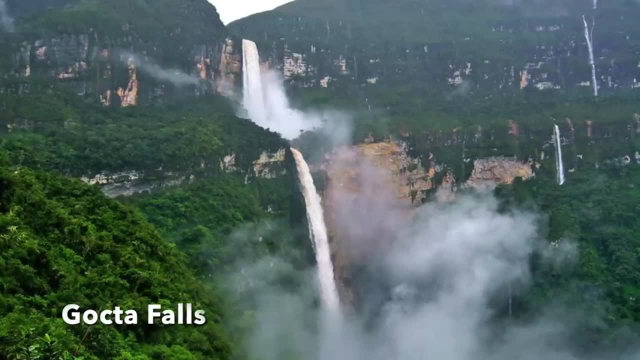 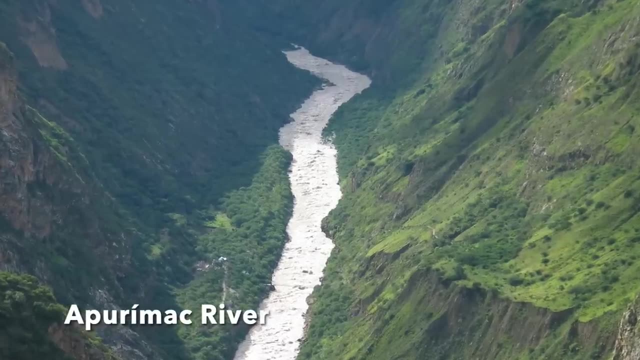 The fifth tallest waterfall in the world, Another waterfall that is somewhere between the third and sixteenth tallest, depending on who you ask and how it's measured- The farthest source of the Amazon River. What other interesting geography facts about Peru did I miss? 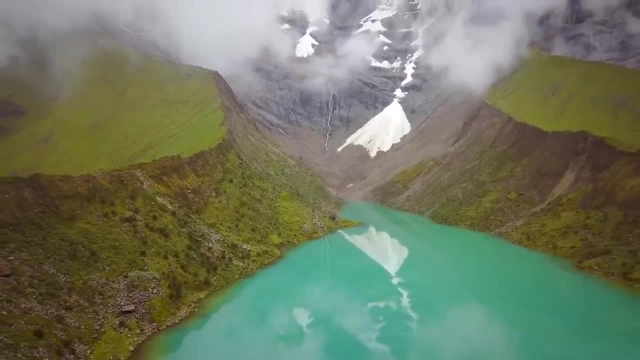 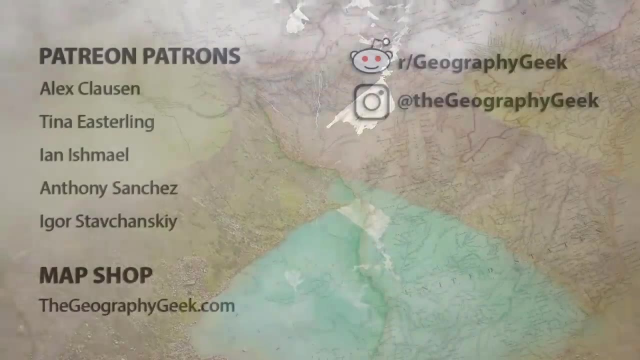 Let me know in the comments below. below. Before I end this video, I just want to put out that every Monday, I send out an email with new content. This way, I can reach people even if the YouTube algorithm isn't working for my videos. 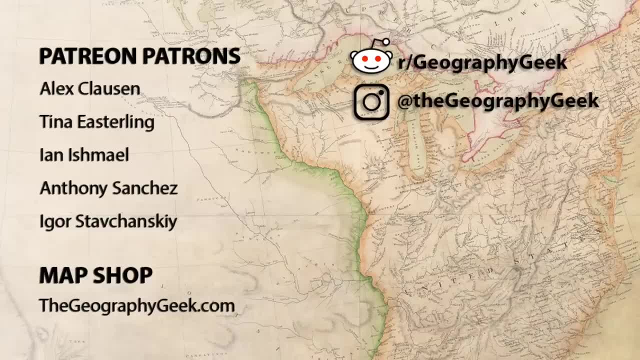 If that's for you, I've left a link in the description where you can sign up. Also, big thanks to my Patreon supporters. If you enjoyed this video, please hit the like button and subscribe for more geography videos. Thank you for watching. Subtitles by the Amaraorg community.